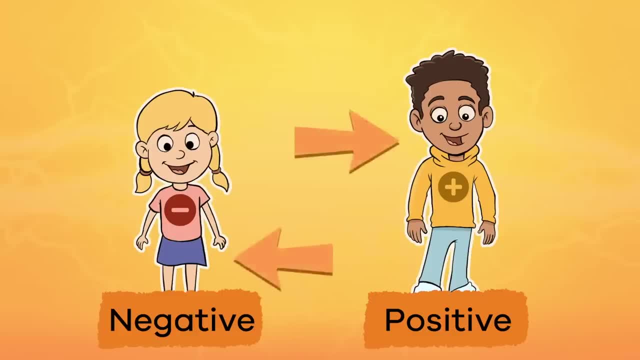 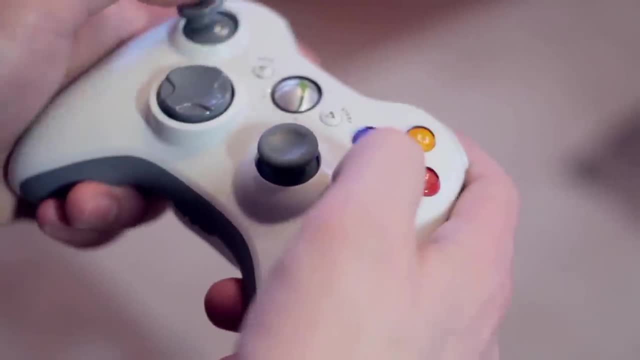 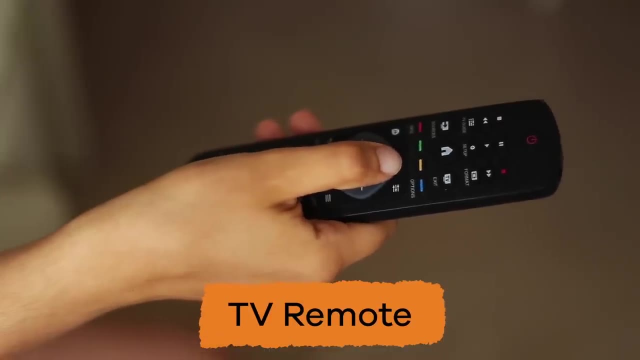 The electric current in the batteries always flows away from the batteries. The electric current in the batteries always flows away from the batteries in the same direction and in a loop from the positive to the negative side. Batteries power things like game controllers, flashlights, phones, even the TV remote. we fight over. 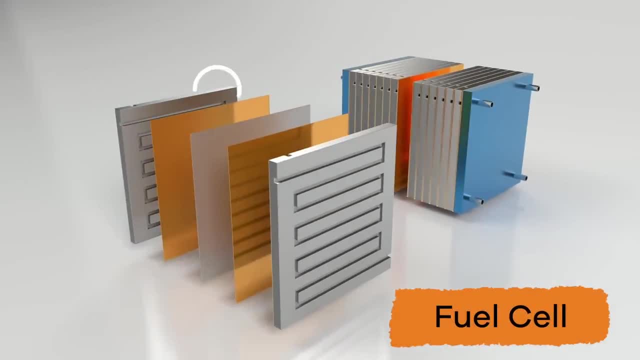 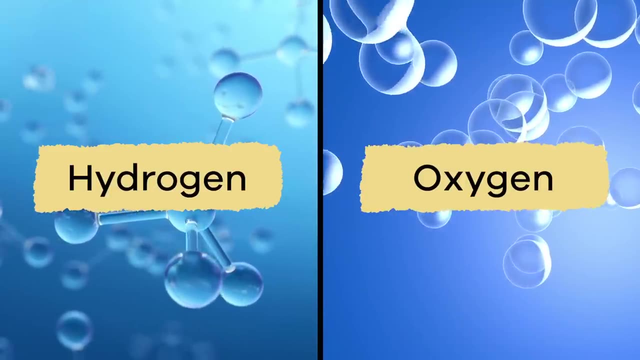 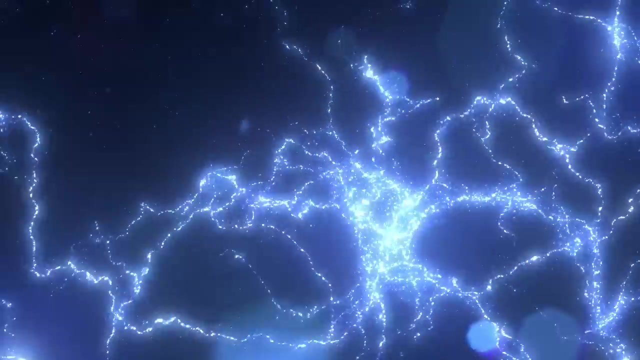 Fuel cells also work like batteries, except they don't need to be recharged. Fuel cells take chemicals like hydrogen and oxygen and put them together. When the two chemicals react to each other or have a chemical reaction, electricity is created. Fuel cells can provide power for something as big. 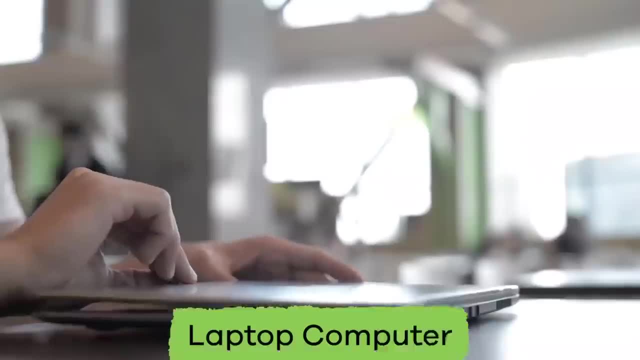 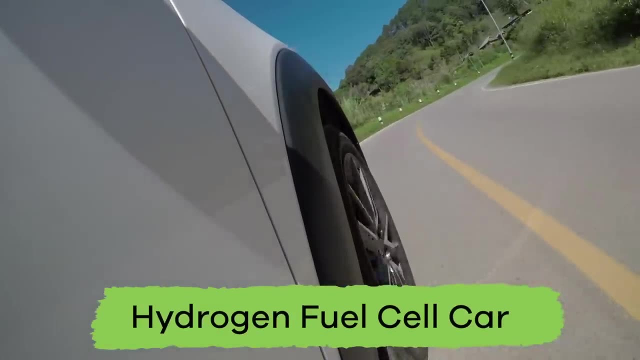 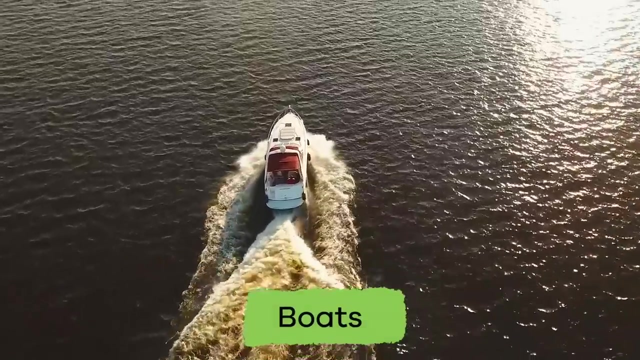 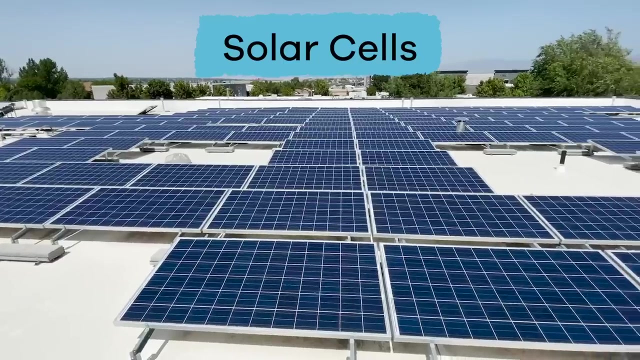 as a utility power station to something as small as a laptop computer. There are even hydrogen-powered vehicles that use fuel cells. Some of these vehicles include forklifts, cars, boats and buses. Have you seen solar cells on the roofs of various homes and buildings? 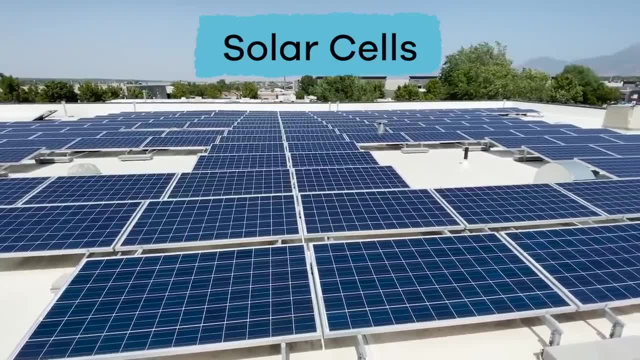 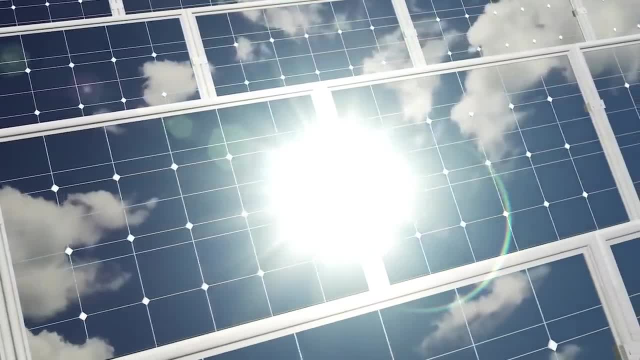 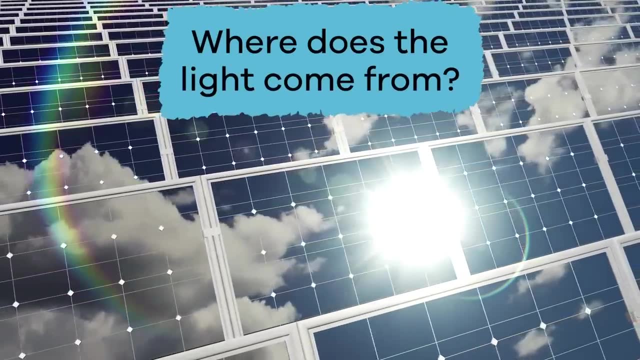 Maybe you even have some on your own home. They look like black rectangles made of glass. The materials inside the boxes release electrons when light shines on them, which then creates an electric current. Can you guess where the light comes from that shines on these boxes? 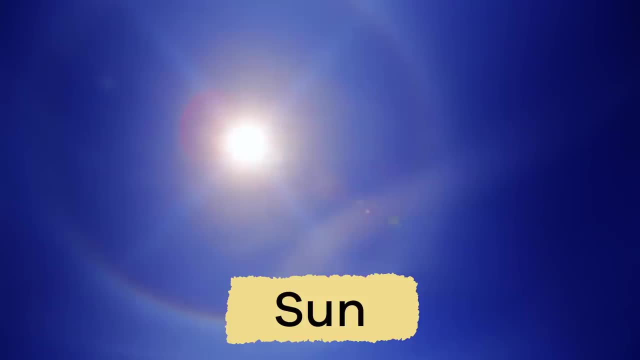 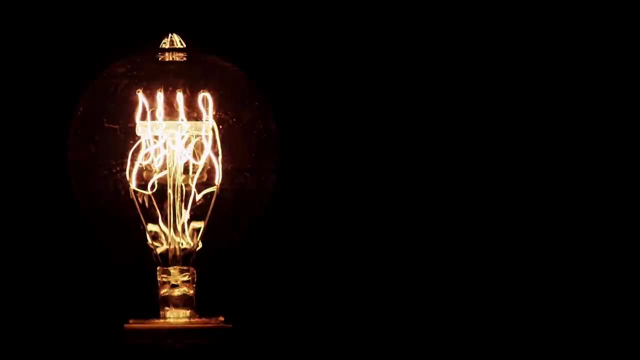 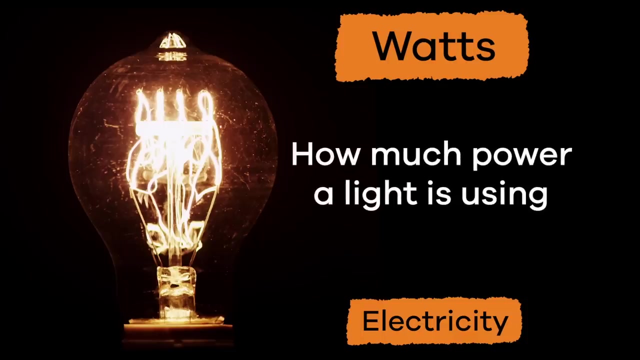 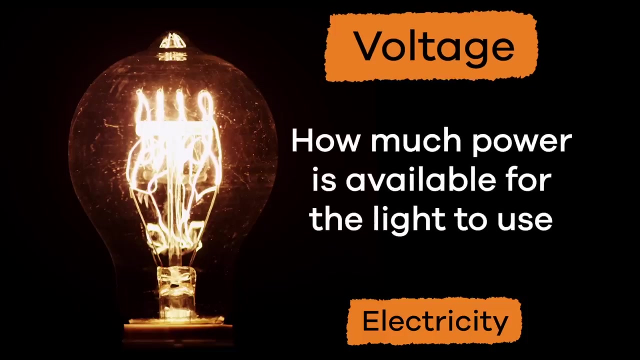 If you said the sun, you're absolutely right. Solar cells use the light from the sun to make electricity. There are some important words that have to do with electricity. These words are: watts, or how much power a light is using. voltage, how much power is available for the light to use. 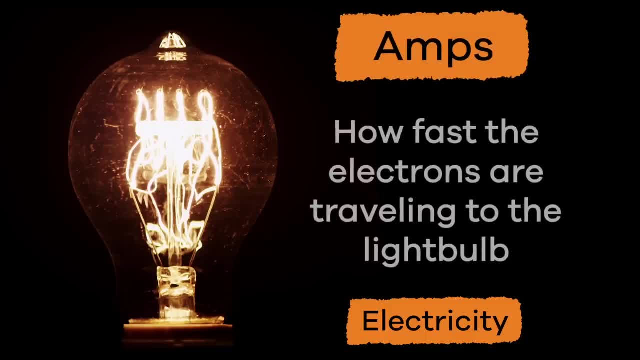 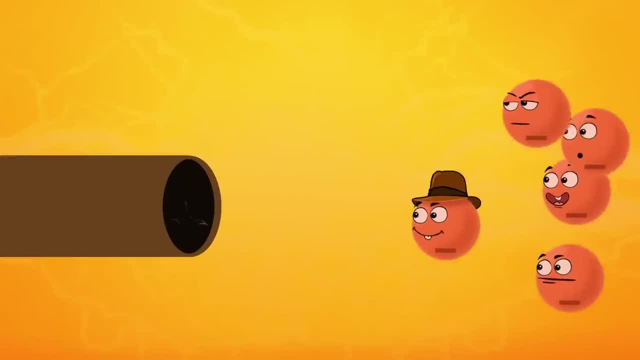 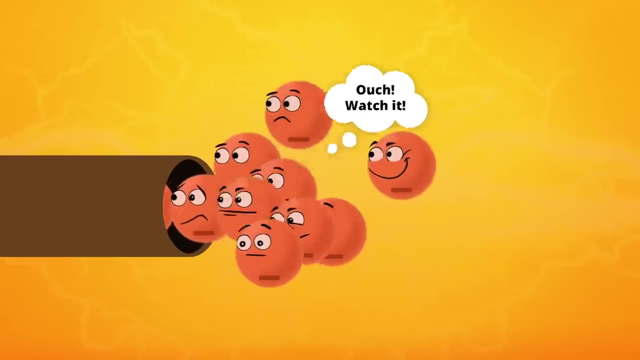 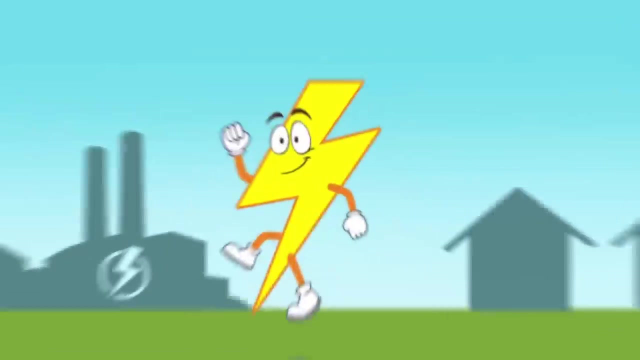 and amps how fast the electrons are traveling to the light bulb. Shorter, longer, thicker and thinner wires also affect how electricity travels. Shorter and thicker wires allow for better flow of electrons than thinner and longer wires. Now let's learn about alternating current. 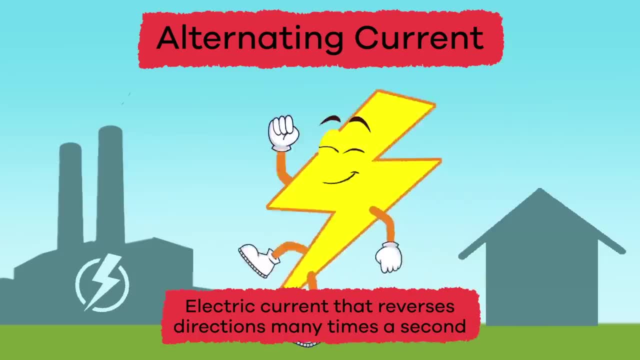 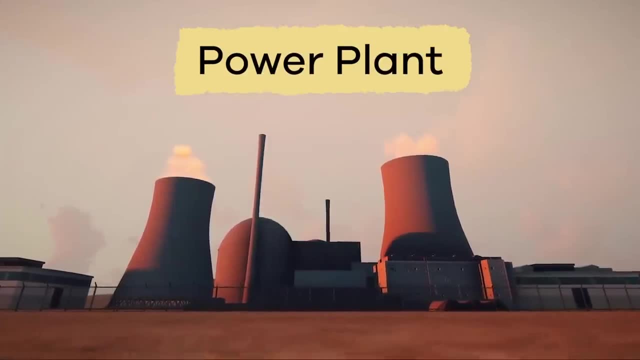 Alternating current is an electric current that reverses directions many times a second. This power comes from the electric current. This power comes from the electric current. This power comes from power plants. The electricity travels through the power lines that you see along roadways and open fields. 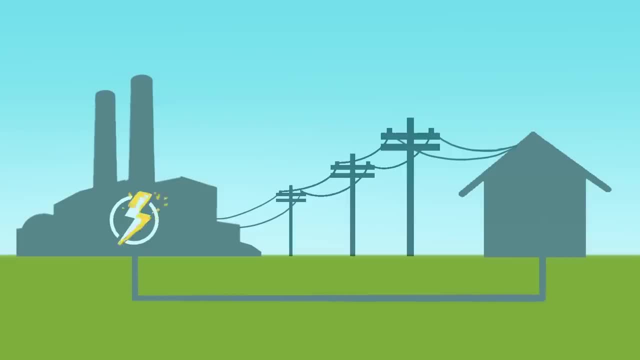 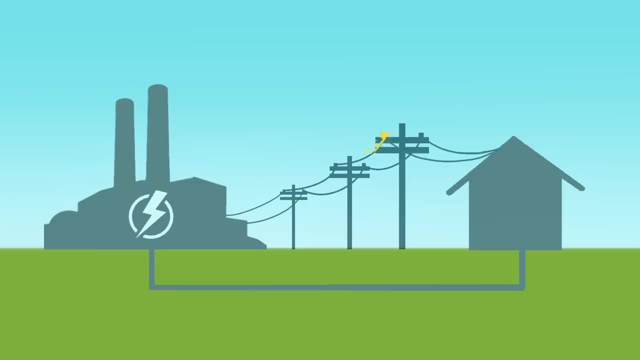 The electrons travel in a big loop from a power plant to the wires that are hooked up to your house, and then back to the power plant again. When you turn on a light in your home or plug something into an electrical outlet, the power flows from the power plant. 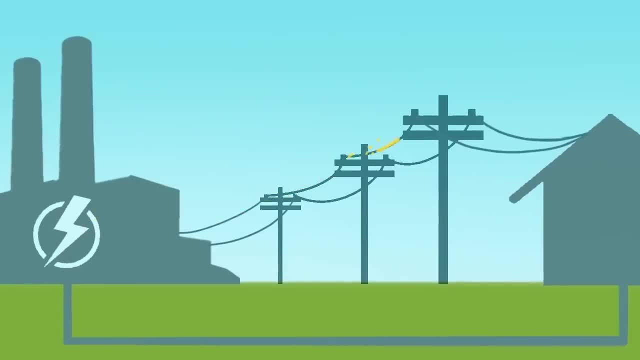 The electronic current travels through these Wrongs to the source B. The electricity travels to your body's base, our body's state of consciousness. When you turn off a lighter and plug your Berlin horn, you do not hear something. but before it enters your home, 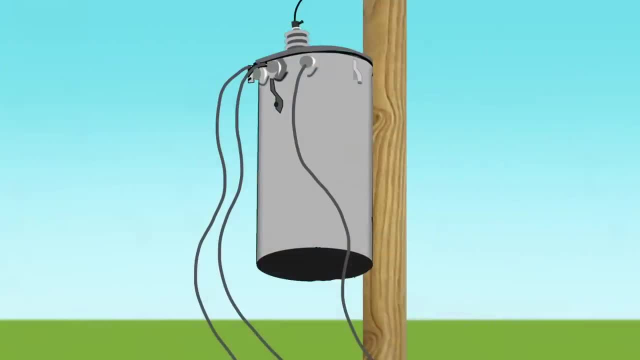 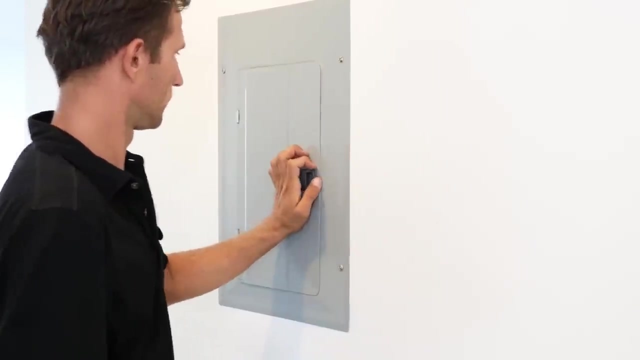 it passes through something called a transformer. Nope, Not that kind of transformer. That would be really cool, though Transformers are attached to the utility box or power poles near your home. The electric current flows from the transformer to the circuit breaker or fuse box in your home. 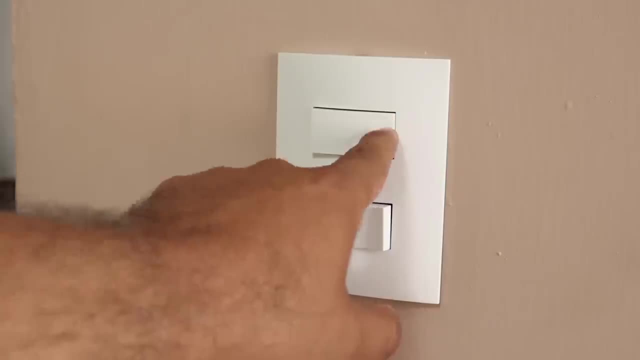 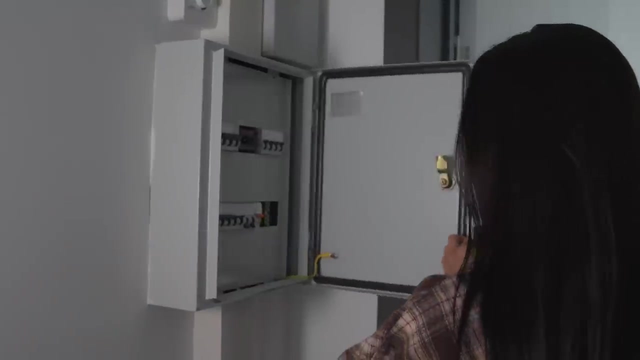 That fuse box then routes the electric current to each of your home, each of your outlets, and switches. The transformer's job is to make sure that the right amount of power is going to your home. This is a very important job If too much electric current flows all at once. 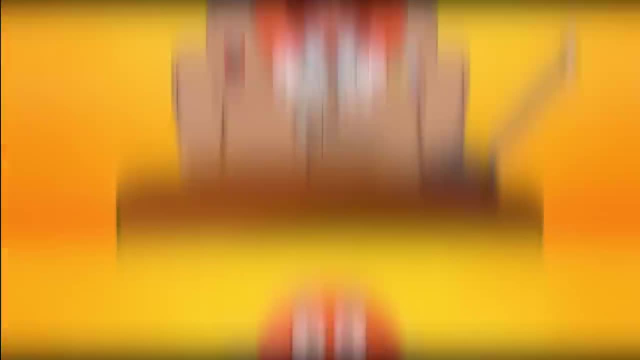 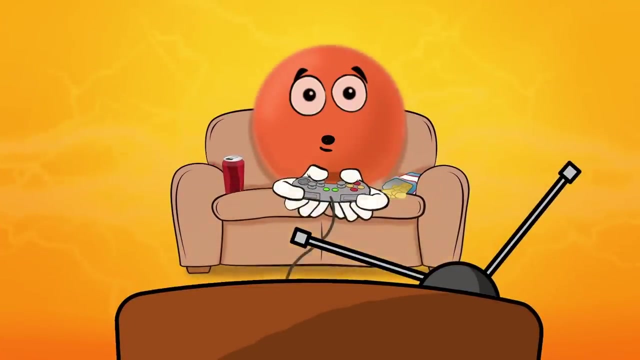 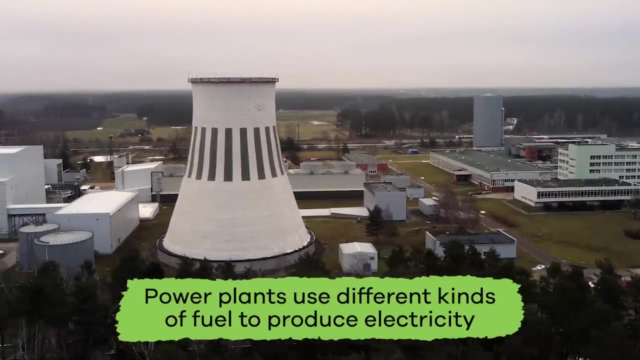 it could blow a circuit and cause all the appliances in your home to stop working, And if too little current flows, it won't be enough to power all of your appliances. Power plants all over the country use different kinds of fuel to produce electricity. 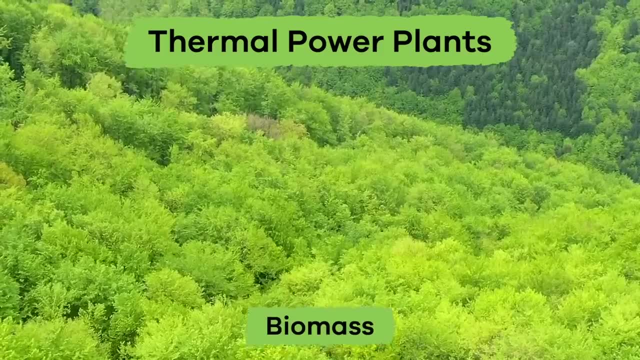 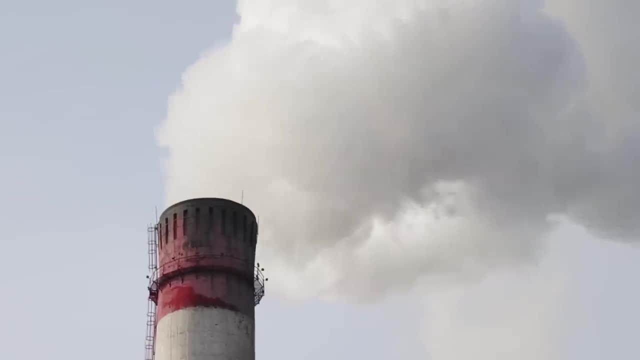 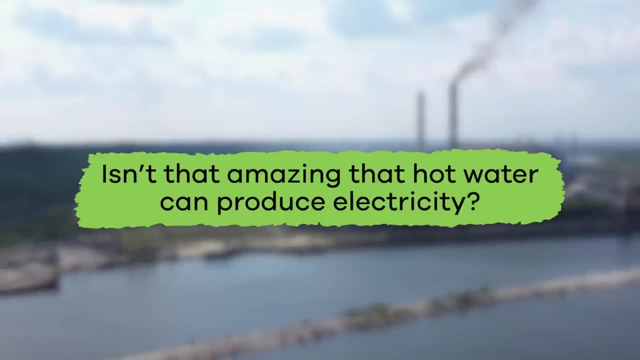 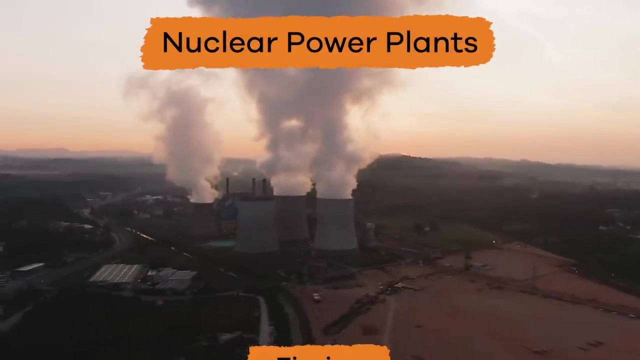 Thermal power plants use coal, biomass, petroleum or natural gas to heat water into steam. That steam then powers a generator which produces electricity. Isn't that amazing that hot water can produce electricity. Nuclear power plants use fission, which means splitting atoms. 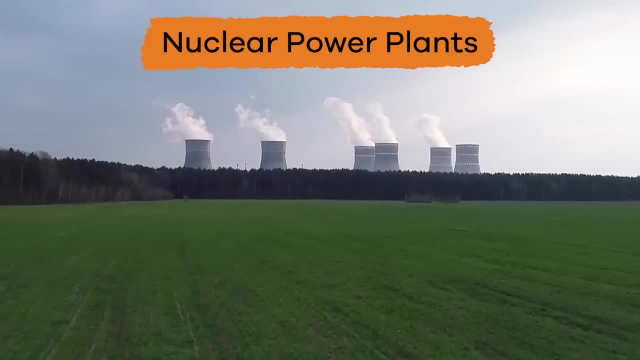 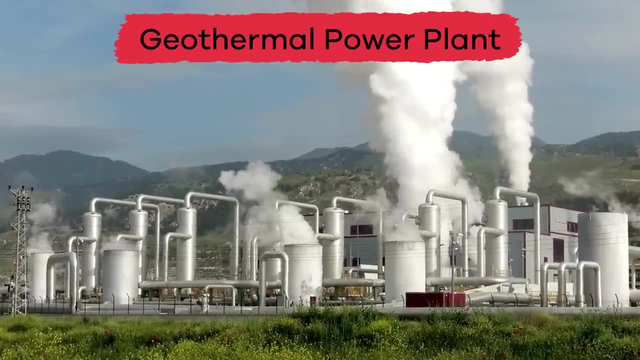 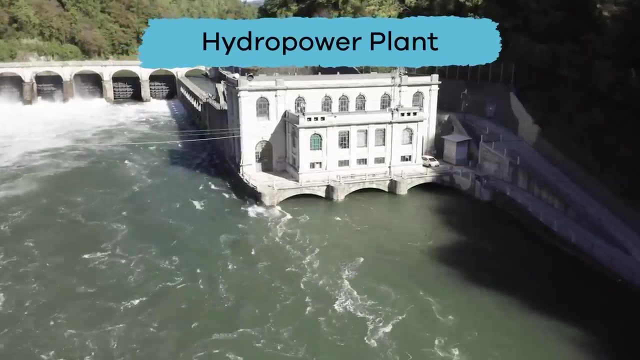 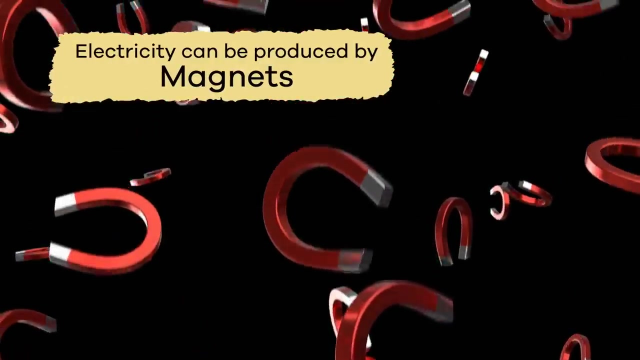 Splitting the atoms creates energy, which produces heat, which also creates steam. Geothermal power plants use the heat located inside the earth to create the steam, And hydro power plants use wind and moving water to create the steam. Electricity can also be produced. 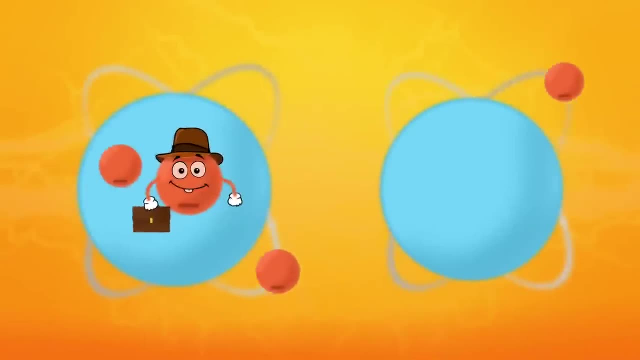 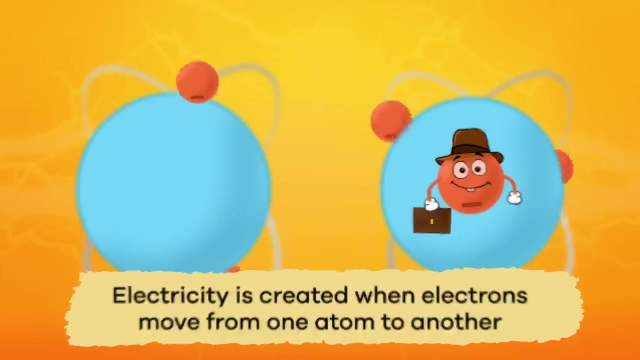 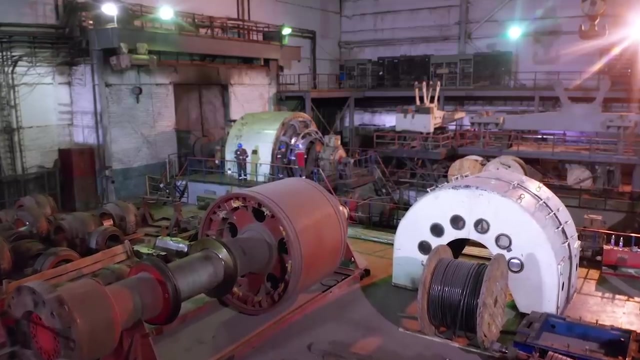 It can be used by magnets. Can you guess why? You already know that electricity is created when electrons move from one atom to another, But did you know that a magnetic field can move electrons? Power plants use giant magnets to create electricity in a generator. 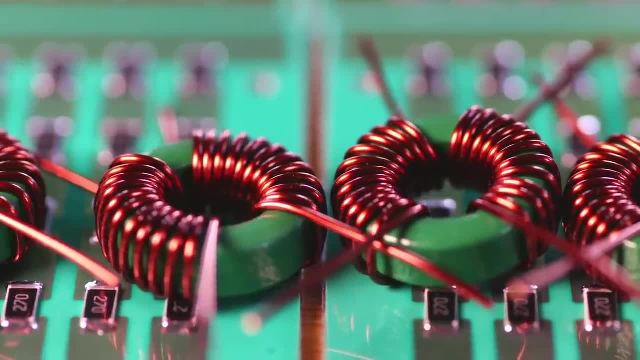 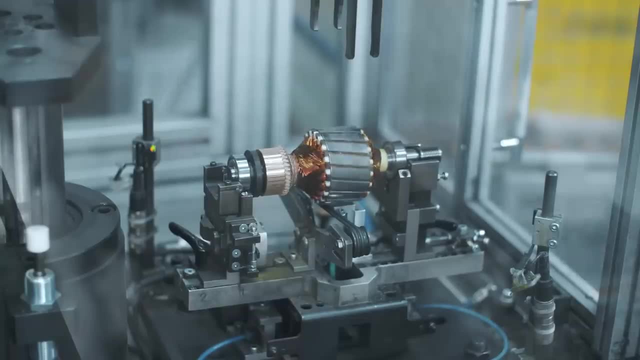 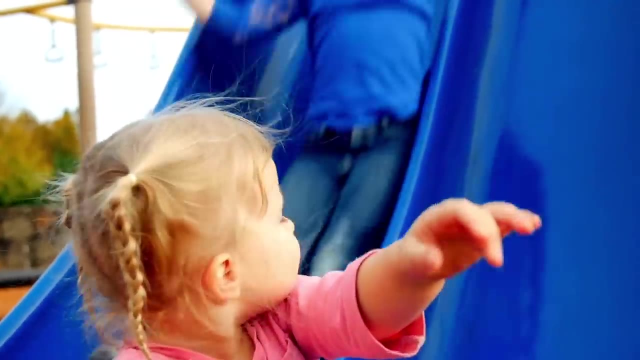 The generator has a coil of copper wire inside the magnets. Steam makes the generator move. It makes the generator spin, causing the electrons in the copper wire to flow through the power lines. Another type of electricity you are probably familiar with is called static electricity. 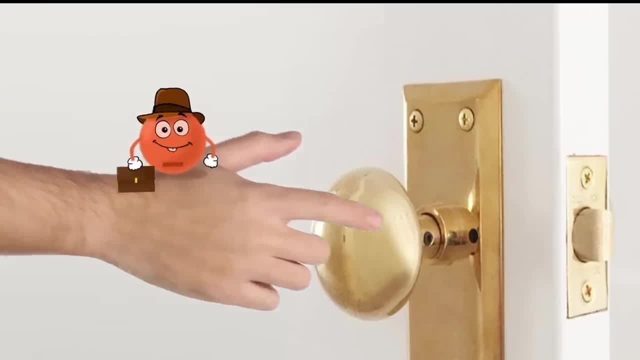 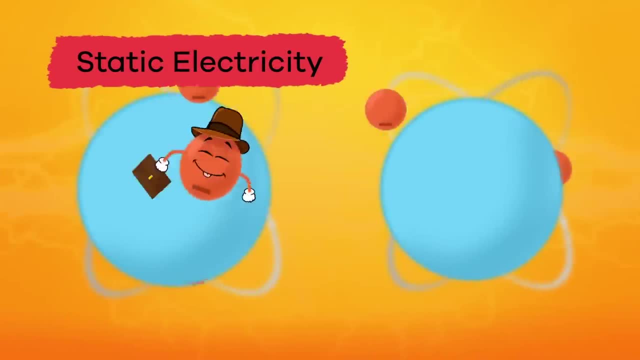 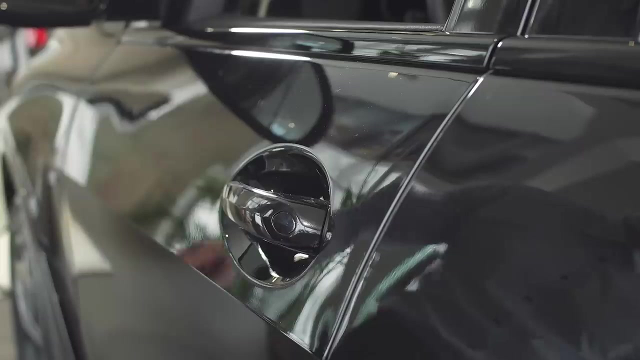 Have you ever been shocked when you touched a doorknob after walking in socks across the carpet? That's static electricity. It happens when electrons move from one place to another, Like from your hand to the doorknob. Electrons can move more easily in some objects than in others. 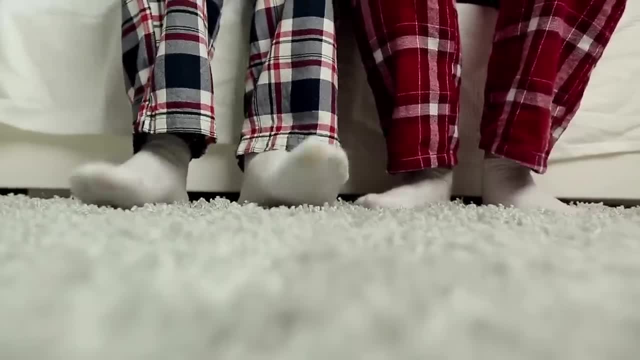 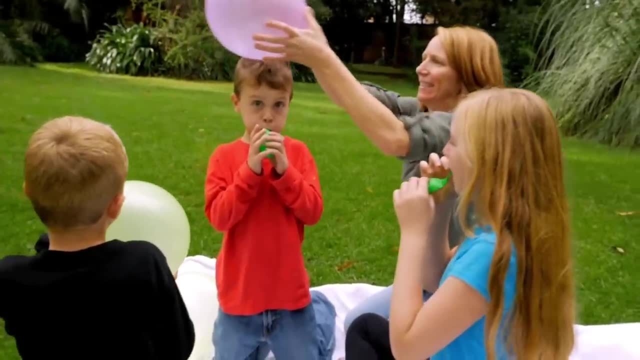 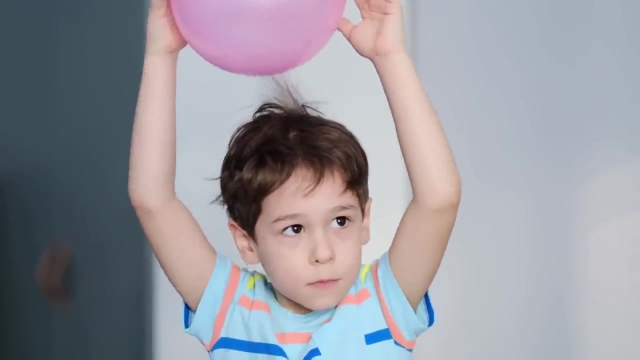 And when certain materials rub against each other, like your socks and the carpet, they transfer electrons. Another example of static electricity is when a balloon is rubbed on your hair. You might have tried this trick before. It's fun. The balloon picks up extra electrons. 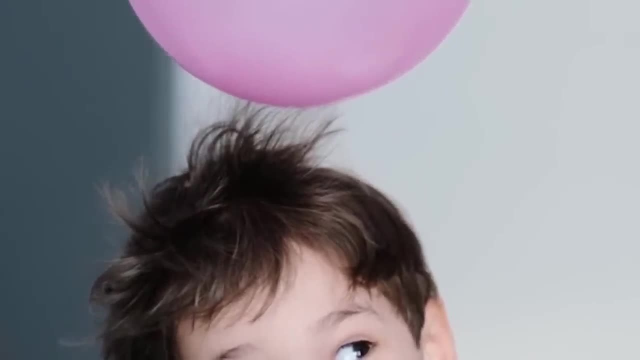 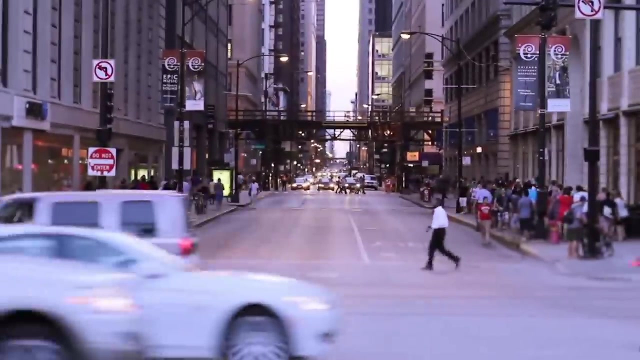 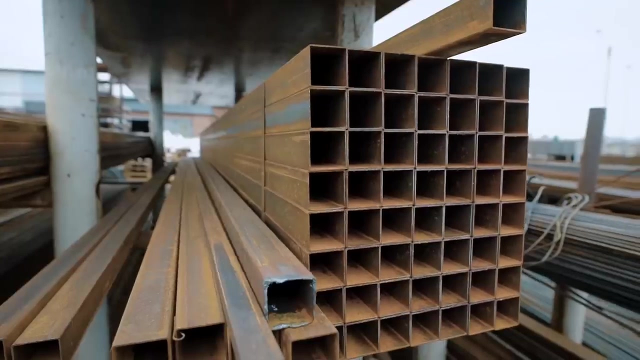 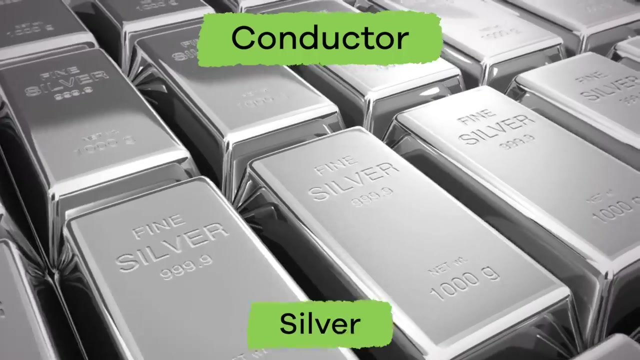 which then attract your hair to the balloon. This causes a literal hair-raising experience. The name for any material or substance that allows electricity to flow through it is called a conductor. Conductors include metals like steel, copper, iron, gold and silver. 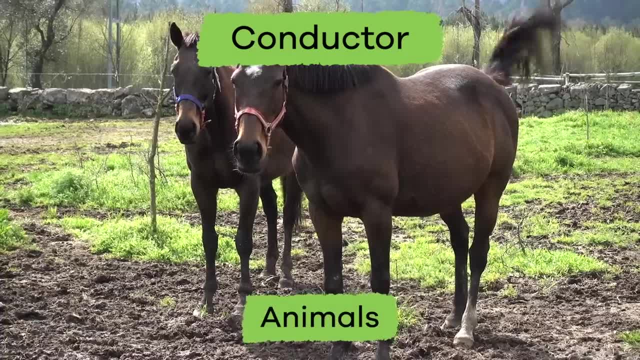 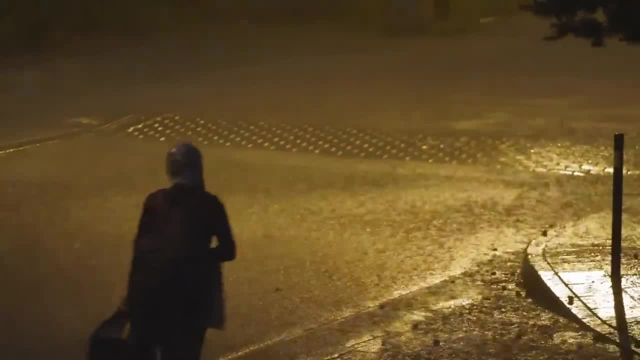 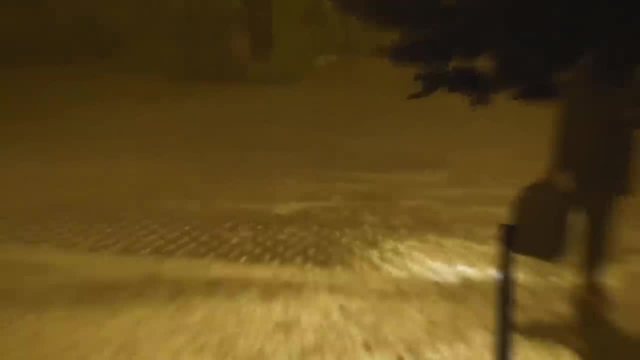 But water, animals, trees and even people can be conductors too. That's why you should stay inside during a lightning storm. You do not want an electric current flowing through you. Insulators, on the other hand, are the opposite of conductors. 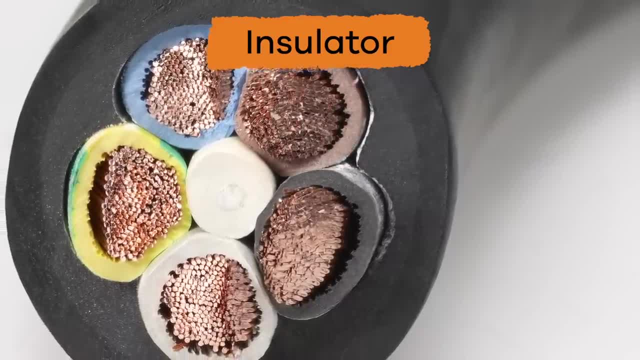 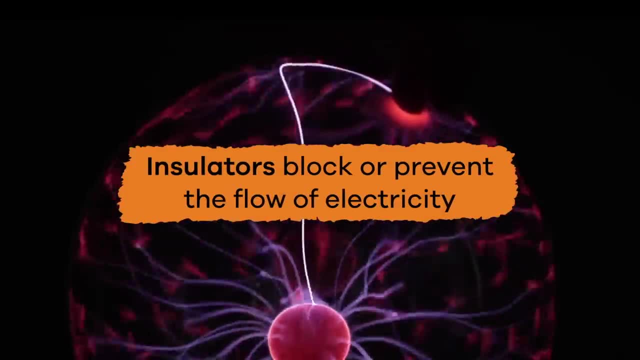 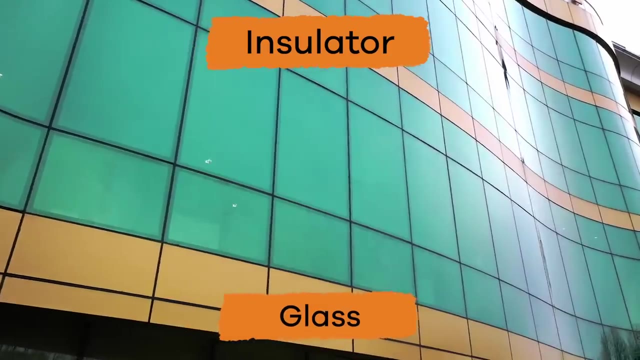 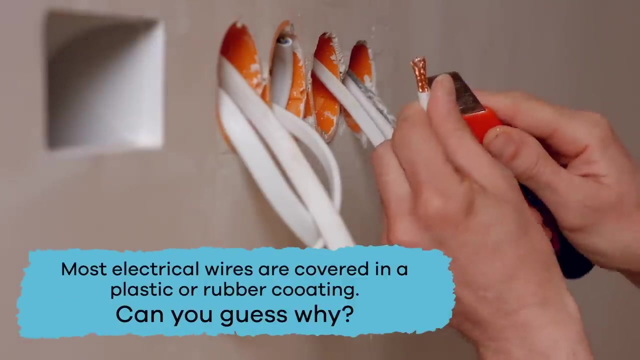 So if conductors allow electricity to flow, then what do you think insulators? do They block or prevent the flow of electricity? Examples of insulators include plastic, glass, porcelain and rubber. Most electrical wires are covered in a plastic or rubber coating. 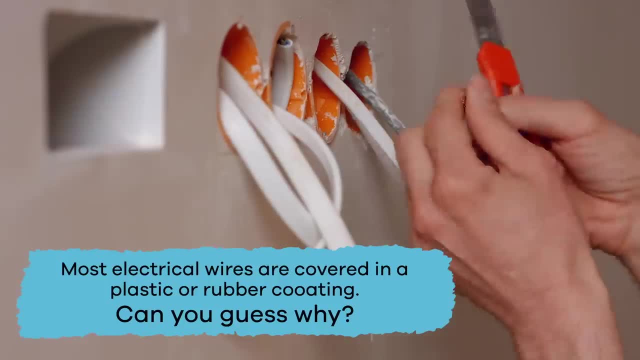 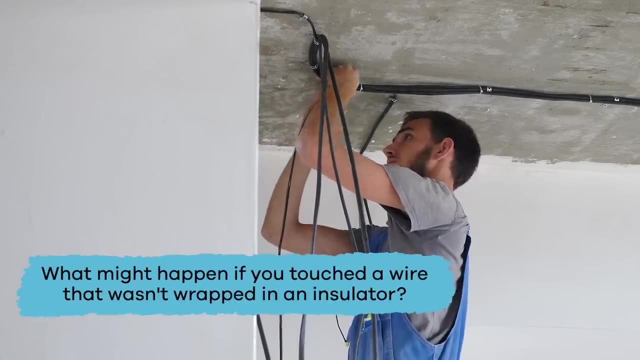 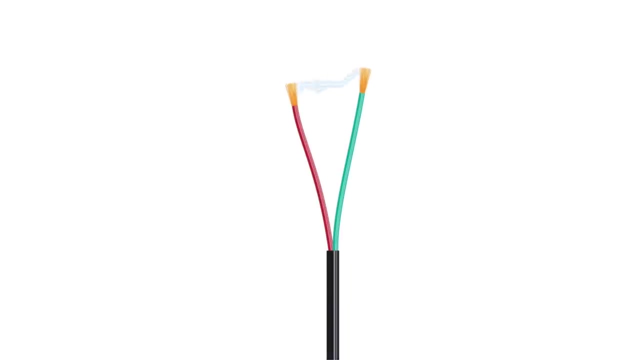 Can you guess why? What do you think might happen if you touched a wire that wasn't wrapped in an insulator? If you said you could get rid of it, if you said you could get shocked? you're absolutely right. It's important to never touch any wires. that you see. 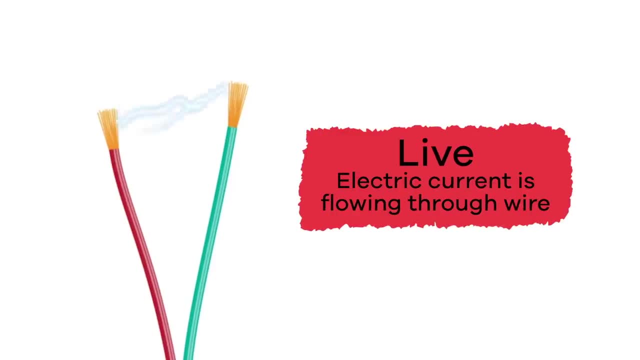 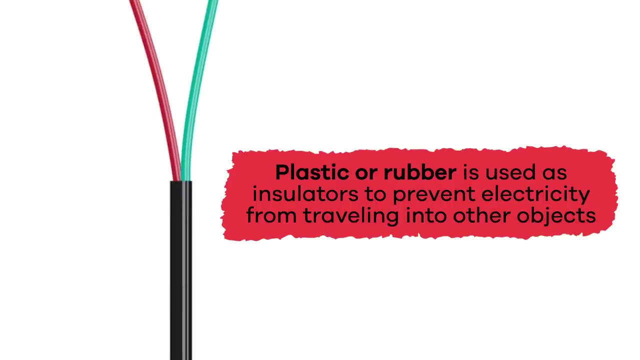 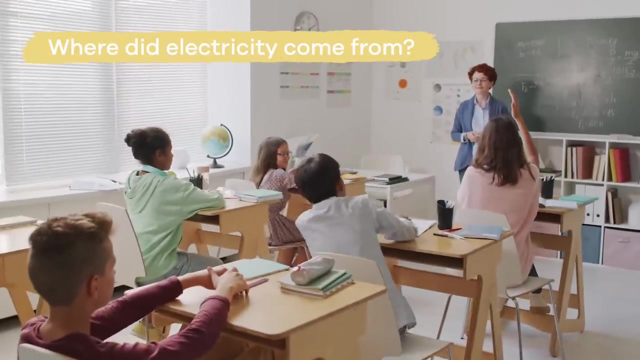 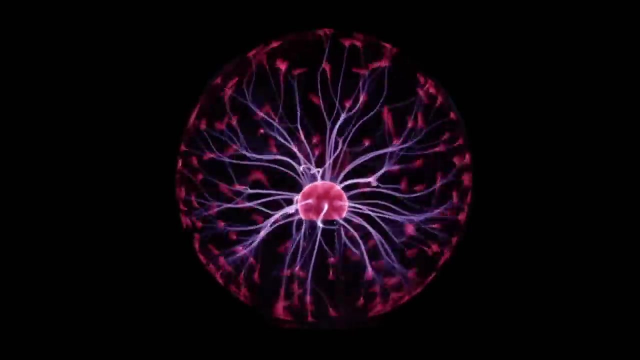 You never know if they are alive, which means that electric current is flowing through them. The plastic or rubber is used as insulators to prevent the electricity from traveling into other objects like yourself. So where did electricity come from? Electricity wasn't invented by anyone. 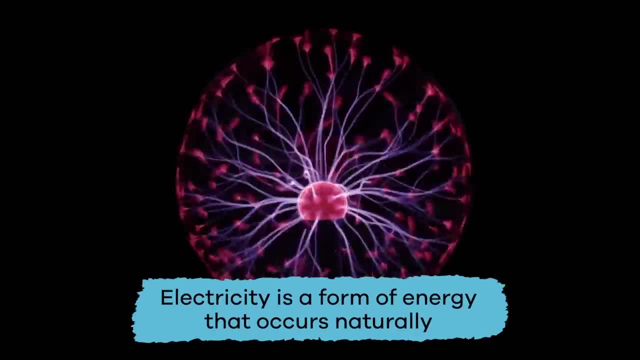 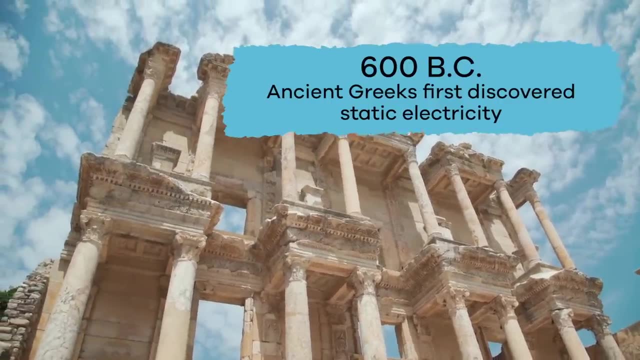 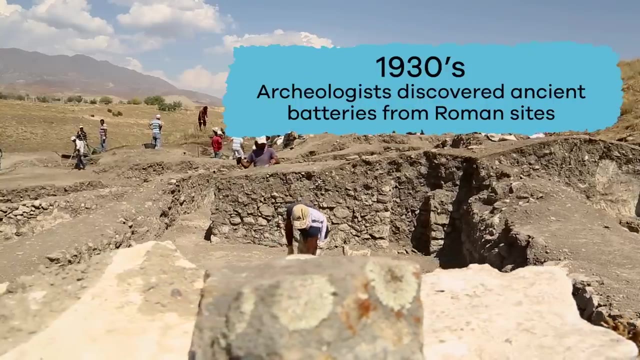 It's a form of energy that occurs naturally. However, it is believed that the ancient Greeks first discovered static electricity in 600 BC, And in the 1930s, archaeologists discovered ancient batteries that may have been used at Roman sites. 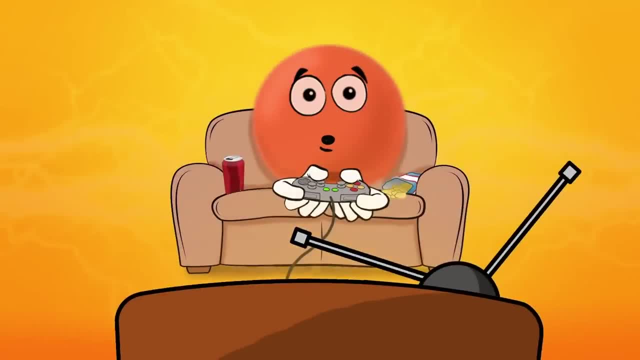 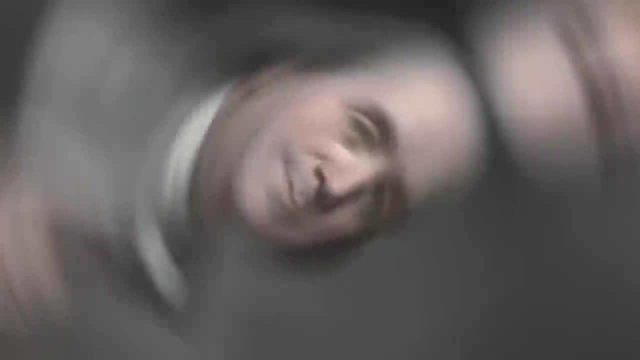 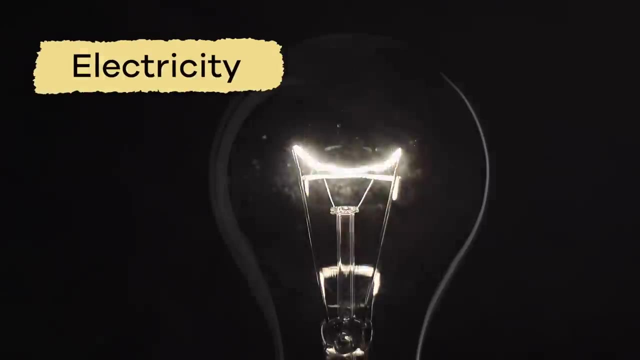 I wonder. I wonder if those would power my controller. People have been doing experiments with electricity for years. You may have seen images of Benjamin Franklin, who was one of America's founding fathers, experimenting with electricity: A kite, a key and a storm. 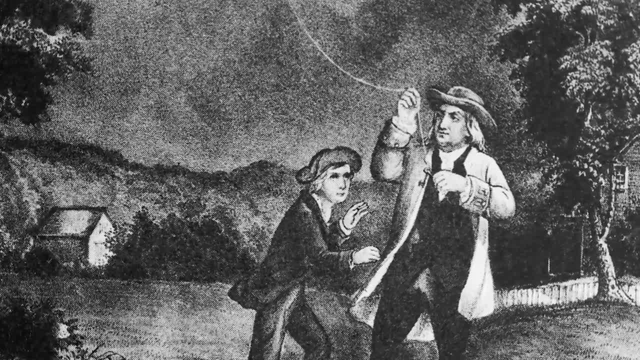 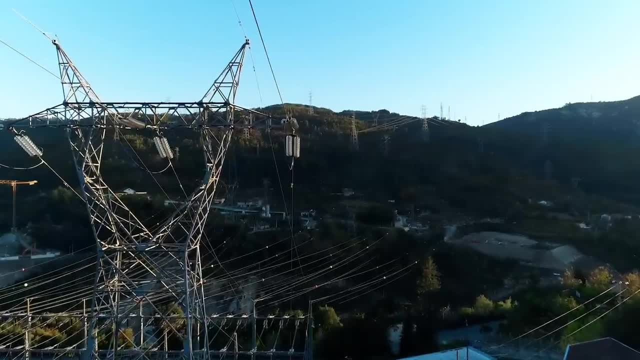 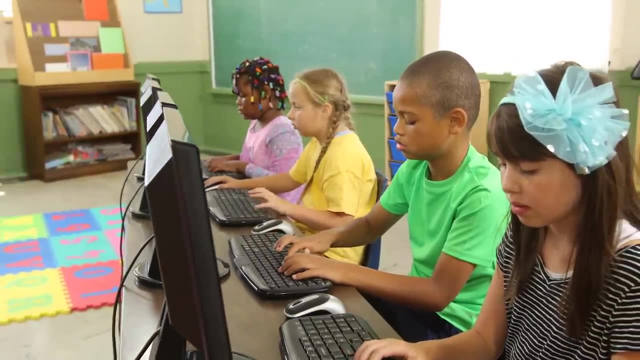 Benjamin Franklin proved there was a connection between lightning and electricity. He was a pretty smart guy. There is much more to be learned about electricity, But what we do know is that without it, life would be much different for many people. Now that you know more about electricity, 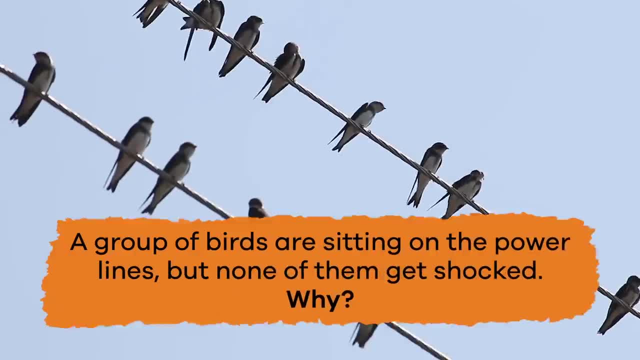 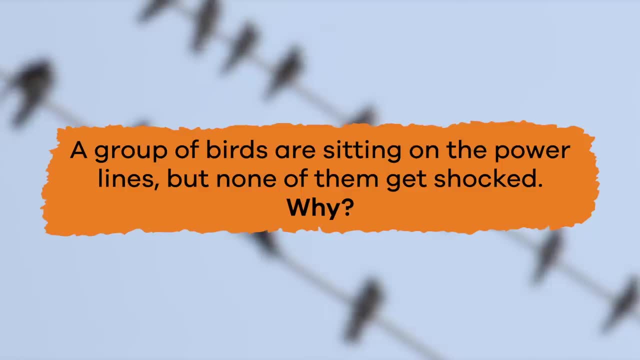 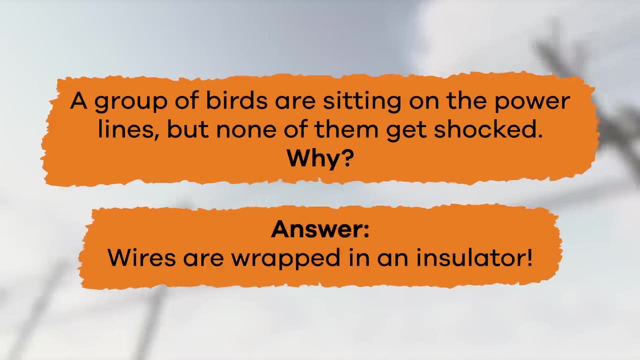 see if you can figure out these riddles. A group of birds are sitting on the power lines near your home, but none of them get shocked. Why? If you said it's because those wires are wrapped in an insulator, you're correct. 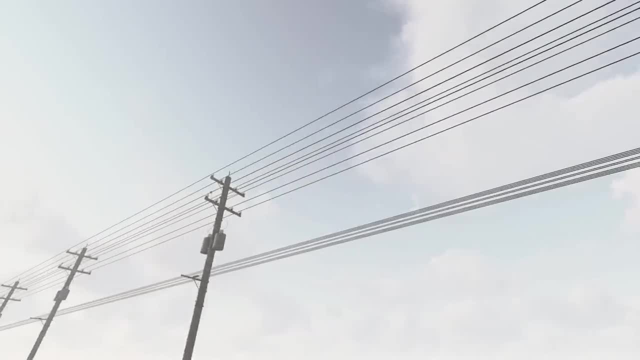 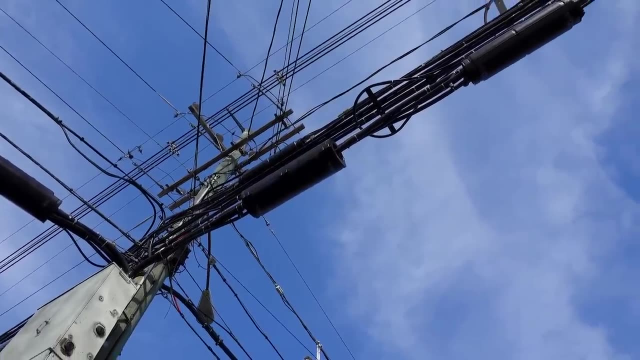 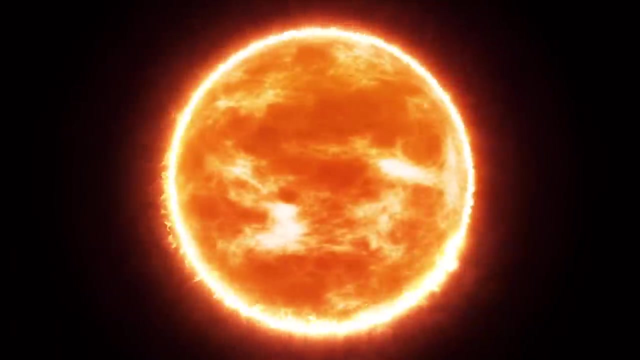 Insulators like plastic and rubber prevent the flow of electricity, But even though they are wrapped, those wires still aren't safe to touch. If you ever see one down on the ground, don't touch it and get a grown-up Ready for another riddle. 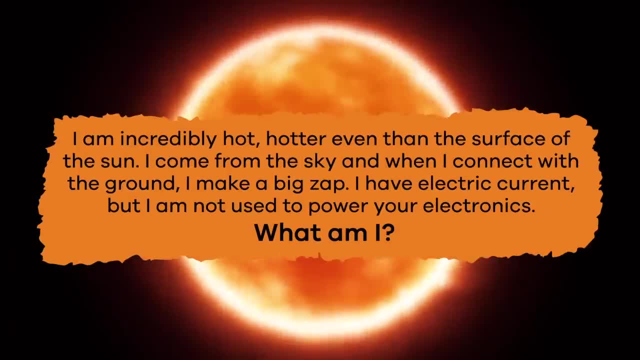 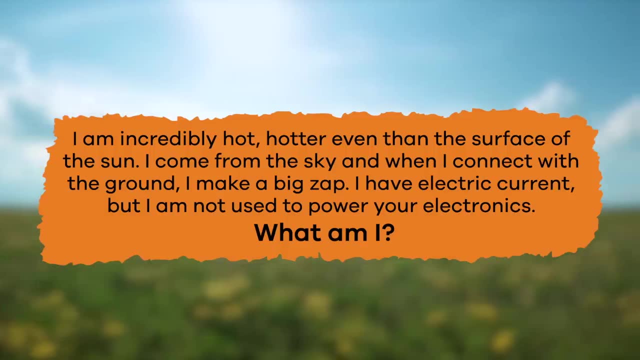 I am incredibly hot, hotter even than the surface of the sky. I come from the sky and when I connect with the ground I make a big zap. I have electric current, but I am not used to power your electronics. What am I? 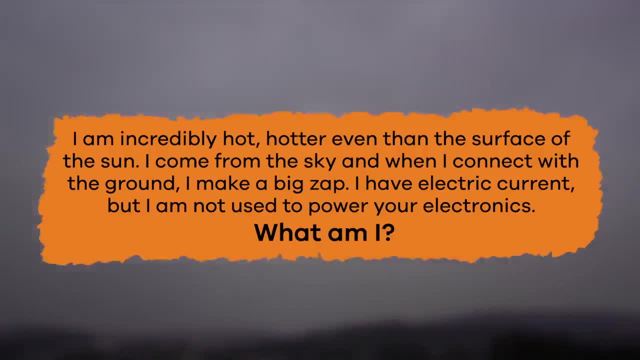 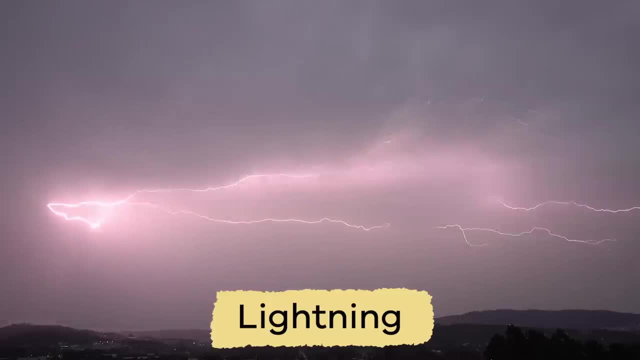 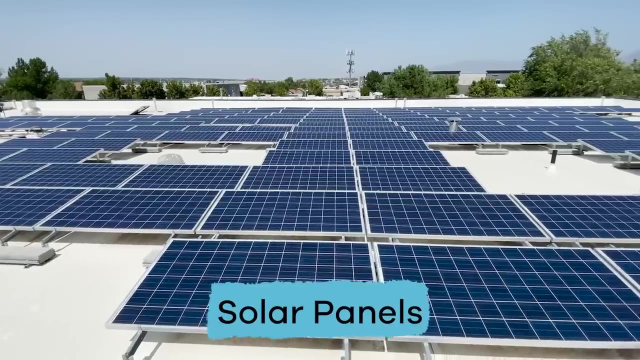 Did you guess? lightning? Well done, Remember. electric current in nature is called lightning and the electric current in our homes is produced by the electric current in our homes. So electric current is produced by power plants, solar panels, batteries and more. 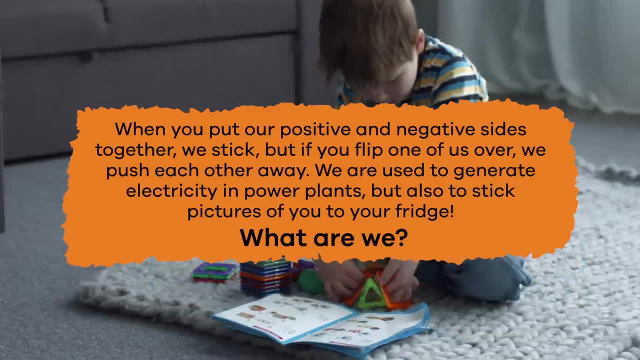 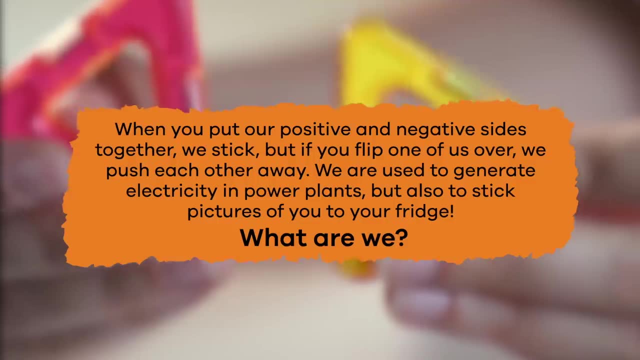 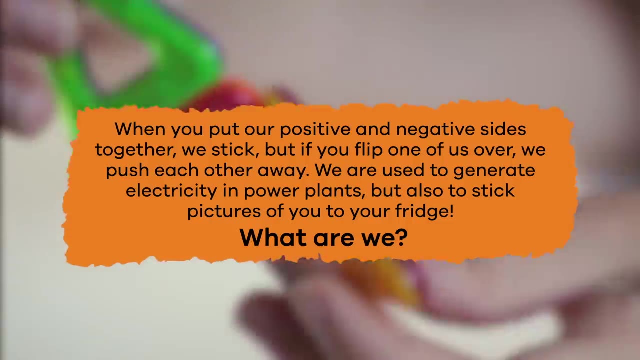 Here's your last riddle: When you put our positive and negative sides together, we stick, But if you flip one of us over, we push each other away. We are used to generate electricity and power plants, but also stick pictures of you to your fridge. 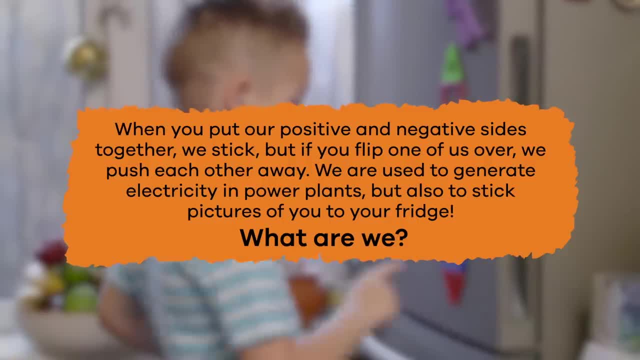 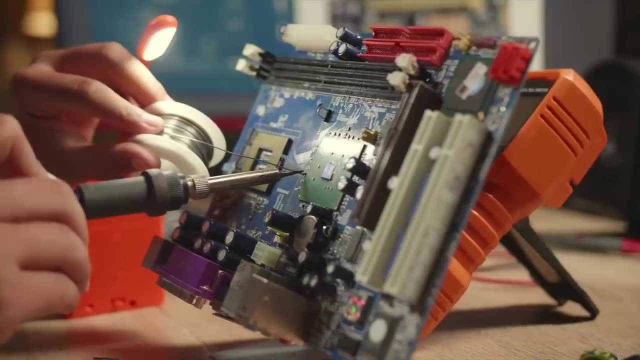 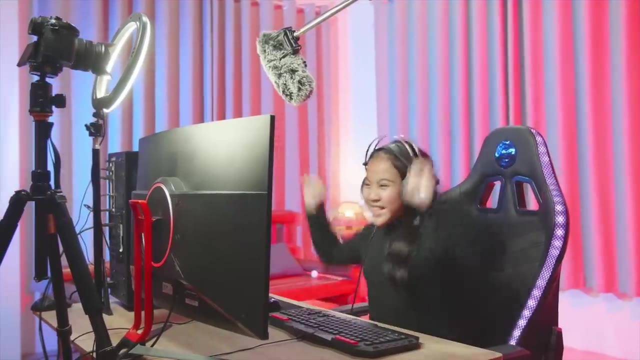 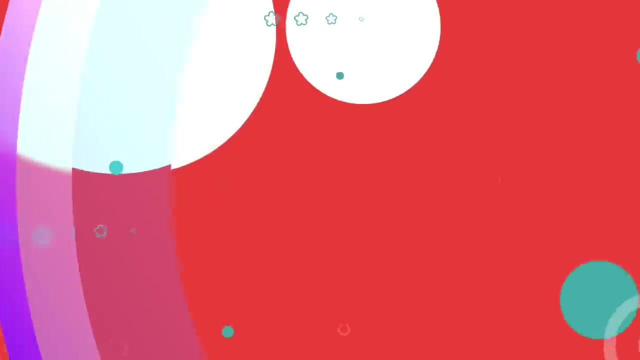 What are we? I bet you said magnets. Well done, Now that you are an expert about electricity, share some of these fun facts with your family and friends. Isn't electricity fascinating? Hope you had fun learning with us. Visit us at learnbrightorg.